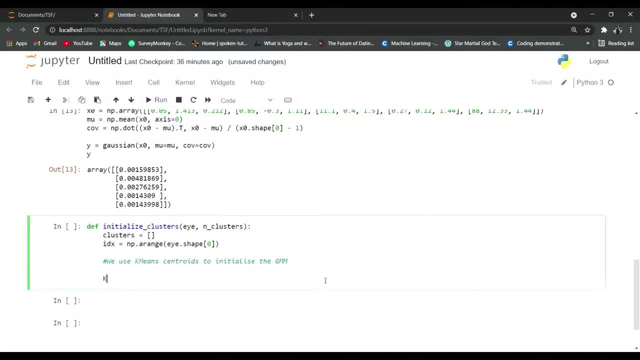 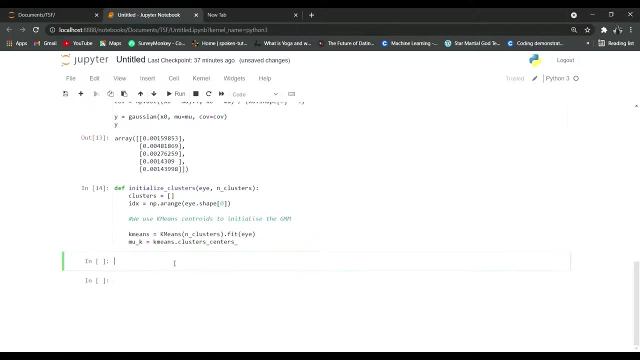 value for mu underscore k and set pi underscore k to 1 over the number of clusters and cov underscore k to the identity matrix. Let's see what went wrong here. Moving ahead to the expectation step, We should now calculate gamma underscore nk. We are giving mu underscore k less than the term sin k multiplied by 1 over the number. 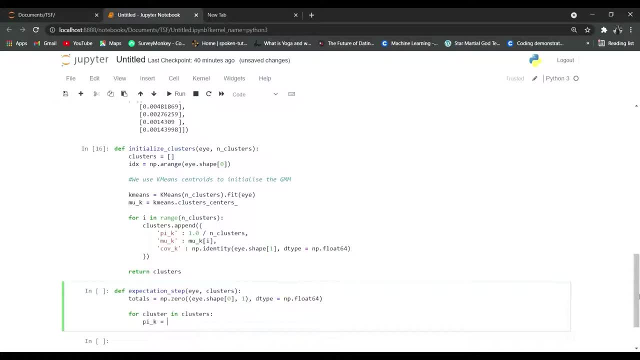 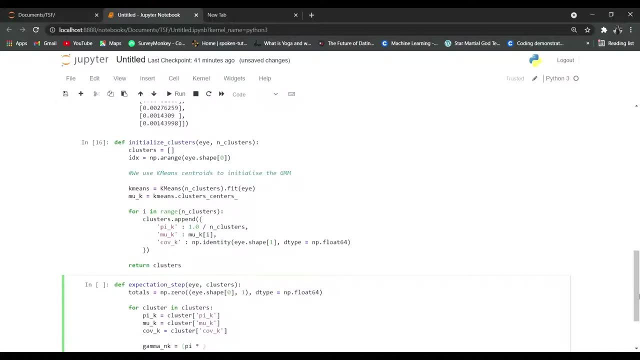 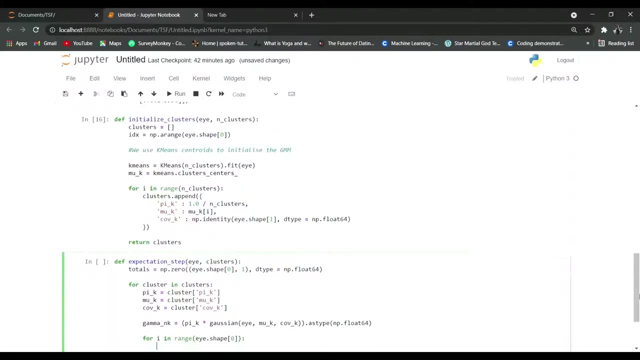 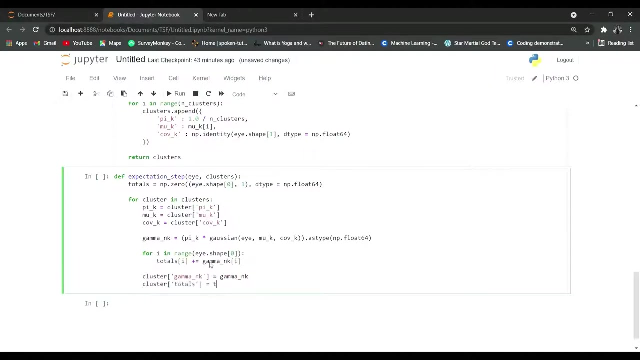 of clusters. We can achieve this by means of the following expression: If the expression to find the gamma underscore, nk or any other, is not clear, you from now eac, the video description for a better understanding of Gaussian mixture model. And now the last part of the experiment: When you memorize a stress problem in bunch of. 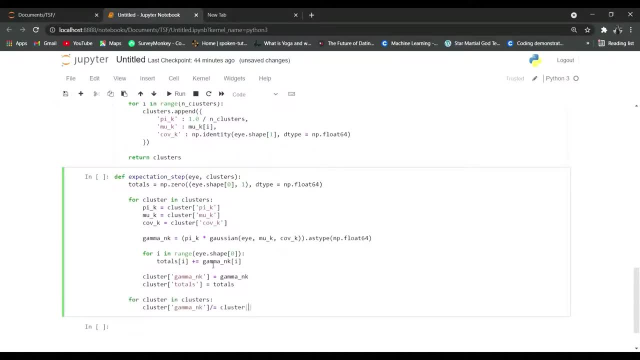 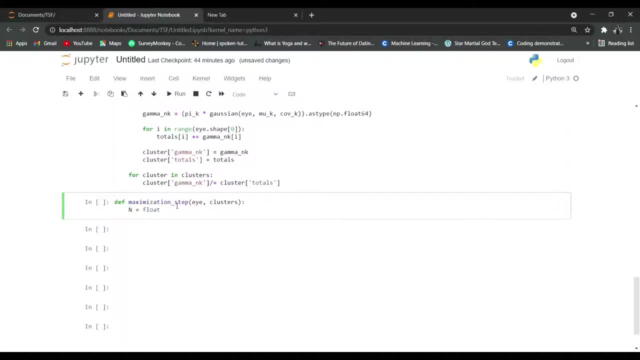 and now the last step: maximization step. let us now implement the maximization step. since gamma and K is common to the expression for PI K, MU K and COV K, we can simply define it and then we can calculate the revised parameters by using the expression given in the code guys note, to calculate the covariance we 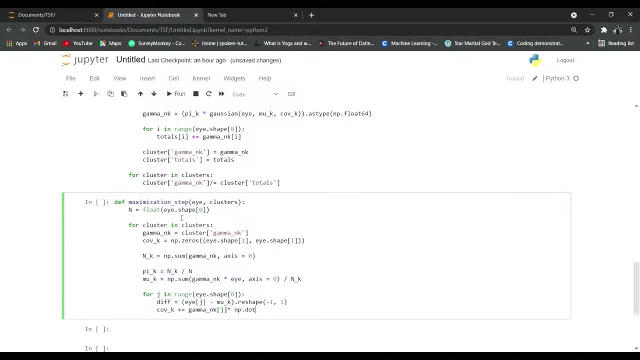 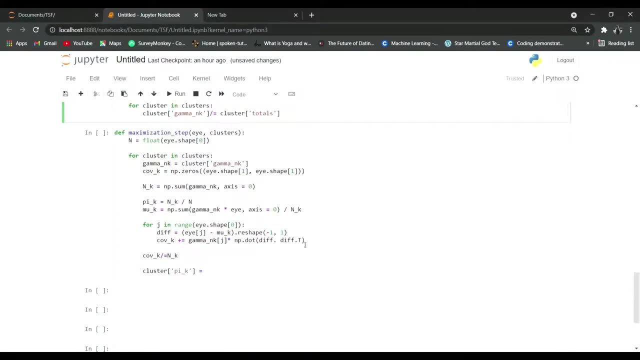 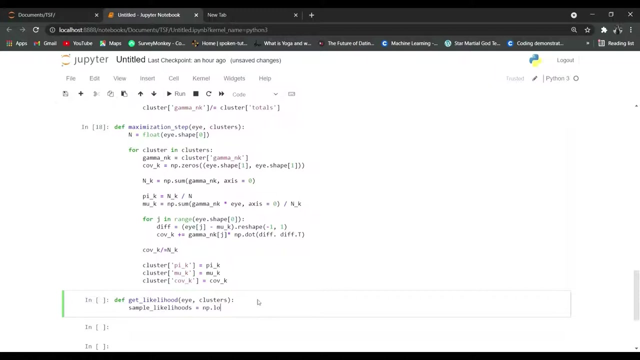 define an auxiliary variable, diff di double F, that contains the given expression. let us now determine the log likelihood of the model. the summation has already been calculated in the expectation step function and is available in totals variable, so we can just make use of it at last. let's work it out. first, we are going to initialize the framework by: 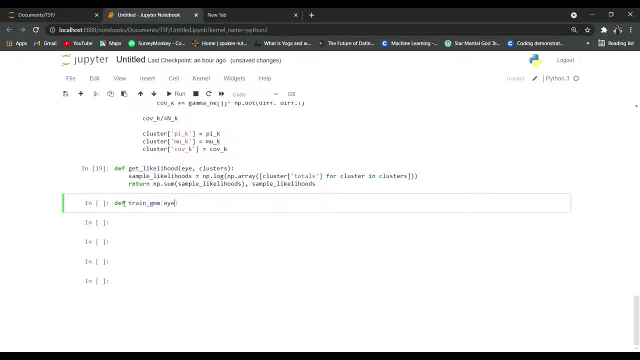 using the initialized clusters and then perform several expectation maximization steps. in this case we set the number of iterations of the training procedure to fix n epochs numbers, so that we can generate graphs of the log likelihood later if we want. the algorithm is motivated by the observation and proceeds. 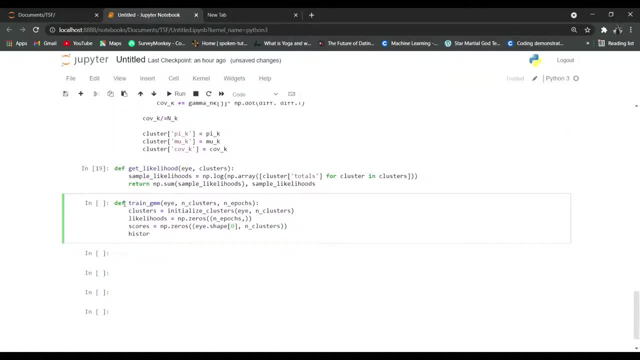 us like initialization of the parameter and evaluating the log likelihood. and then it goes to expectation step no and evaluates a posterior probabilities using the current values and the maximization step. estimates new parameters with the current values. the log likelihood with the new parameter. estimates If the log likelihood has changed. 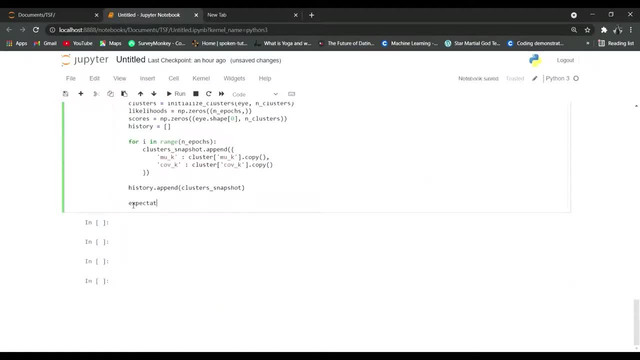 by less than some small value, we can stop. Otherwise we can repeat the expectation step. Note, guys: EM algorithm is sensitive to initial values of the parameters, So care must be taken in the first step. However, assuming the initial values are valid, one property. 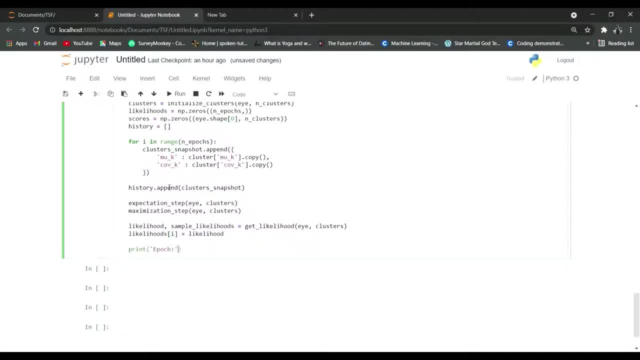 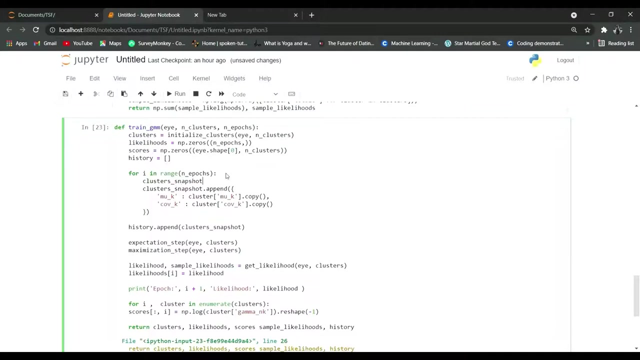 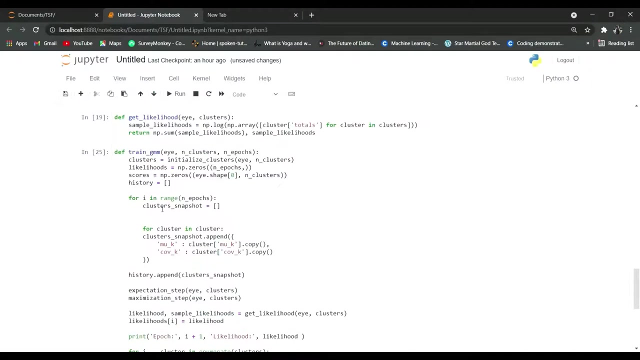 of the algorithm is that the log likelihood increases at every step. This invariant proves to be useful when debugging the algorithm in practice. Something's wrong. Let's check what it is. I have missed quite a few steps here. Damn the indentations. 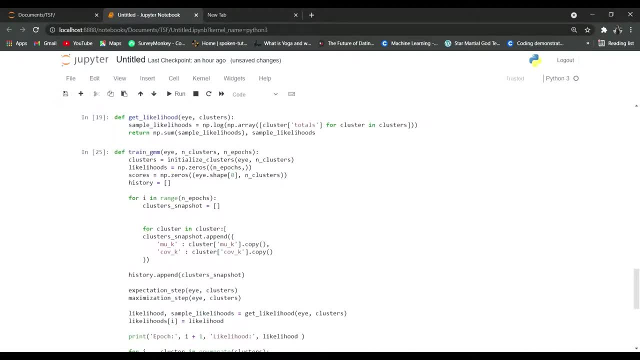 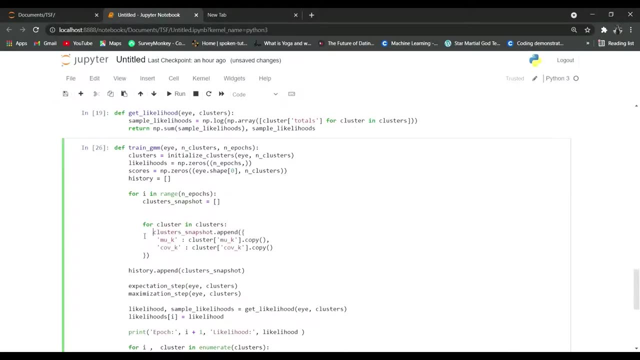 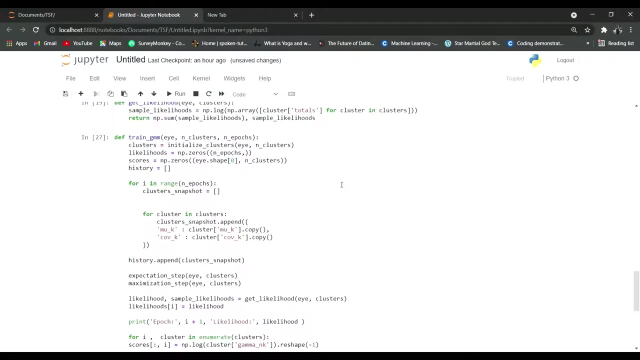 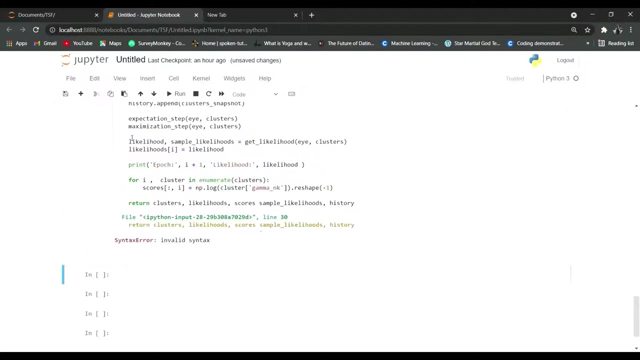 It always takes time to find the errors. Now that we have fixed the errors, let's move ahead: Giving fixed values for yen epox and yen cluster- to train the data, and now we are going to create a graph to visualize our clusters, as well as a framework. 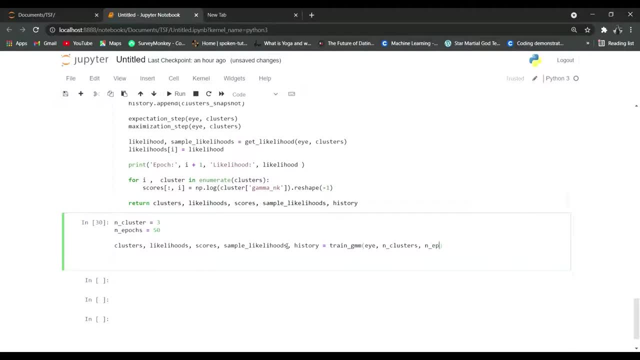 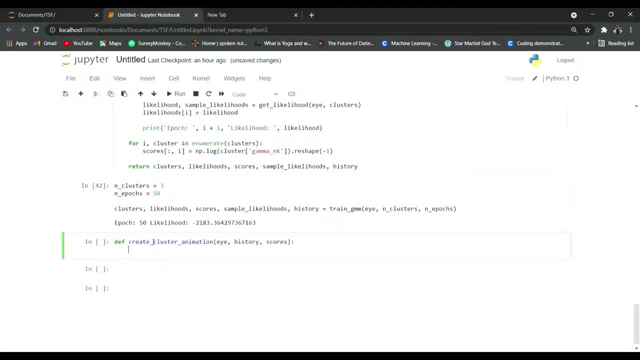 for the gaussian mixture. so what we are going to do here is create ellipses of different scales in order to map to the coordinates of each gaussian. so, so, so, so, so, guys, don't skip the matrix chapter in your school or college, especially the part where 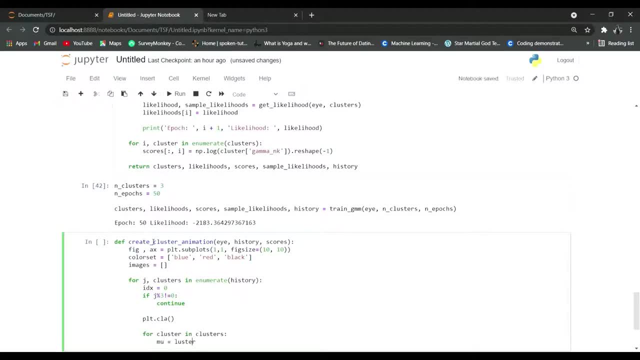 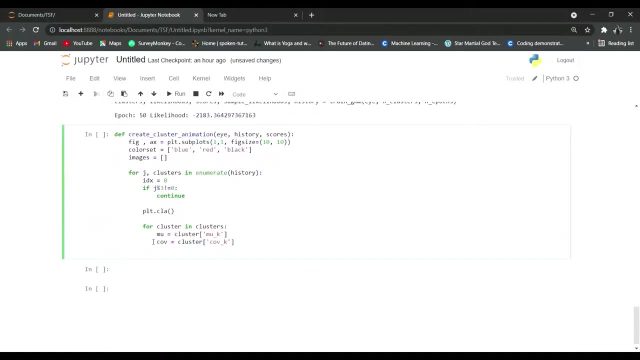 they teach you about eigenvalues and vectors. i did that mistake and i had to learn it again from the go. so guys, don't skip the matrix chapter in your school or college, especially the part where they teach you about eigenvalues and vectors. now let's give the expressions for covariance factor. 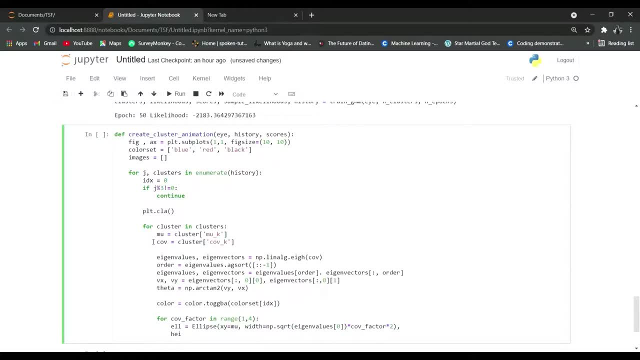 the angle of the ellipse is determined by the covariance of the data and we adjust the value of the covariance to see the data is correlated or uncorrelated, so which results in an axis aligned error ellipse. so it should be clear that the magnitudes of the 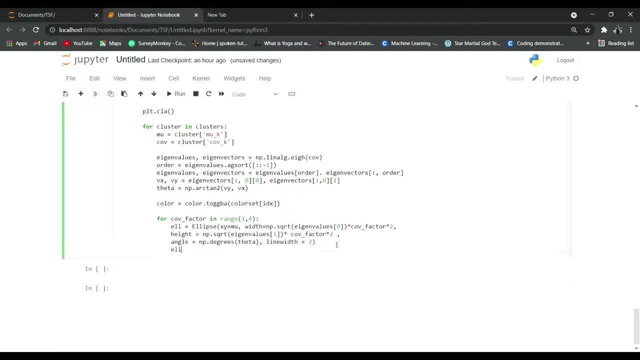 ellipse axis, you know, depend on the variance of the data, and our data is a multivariate gaussian. this means that both the x values and y values are normally distributed to- let's use a matplot, so so the length of the over networks x and y will be the cross results. looking atresponse, 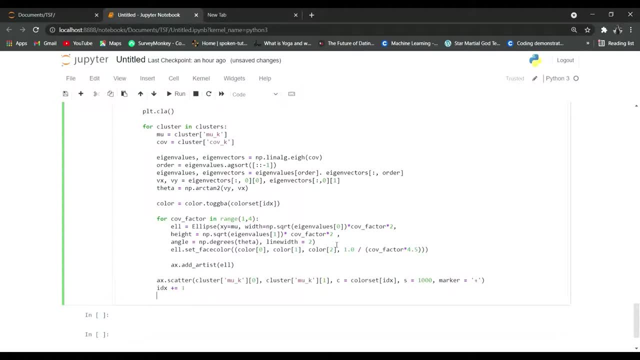 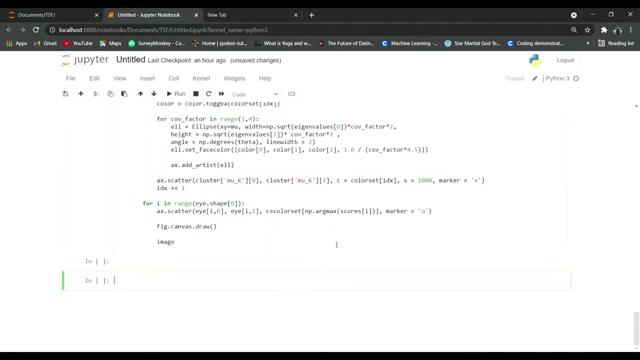 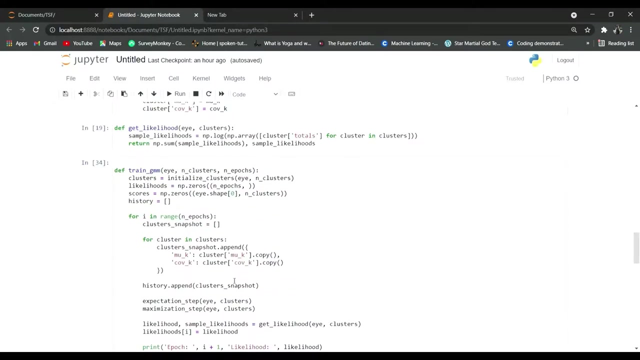 verticals and the Este sine sweep will become less than the over coefficients or the midpoint in the verticals z, p, v. that fills andoro, f n. so Thank you, Error And it's fixed. We can now view the error. LF, also known as confidence LF. 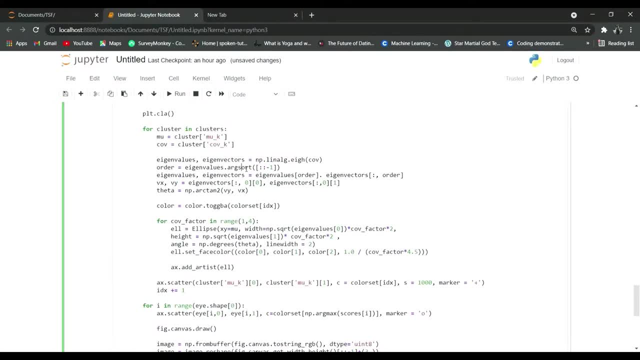 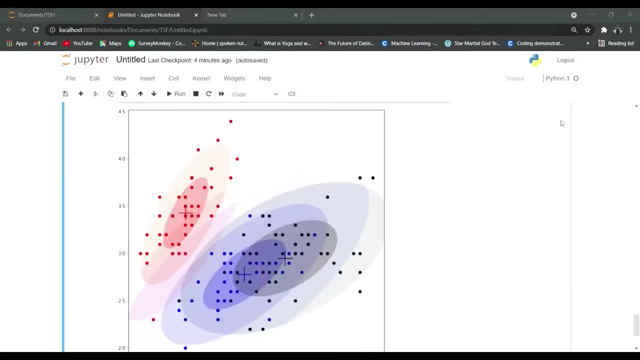 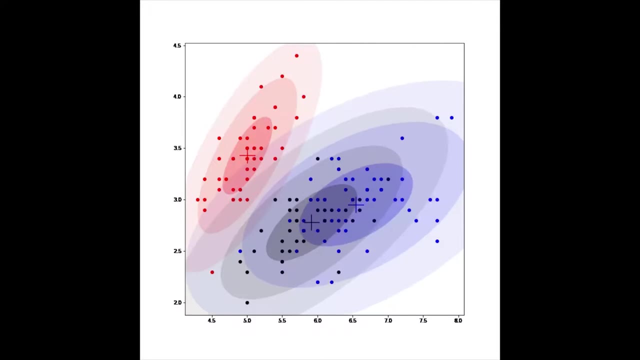 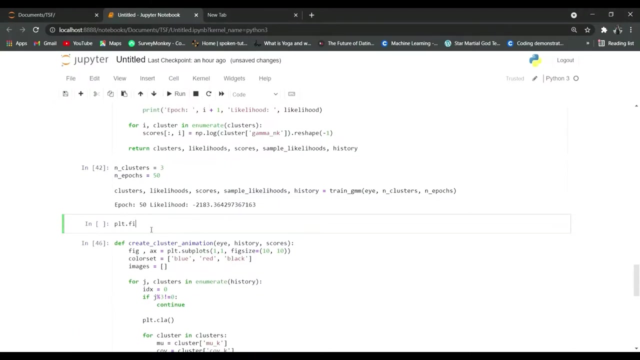 and the animation of how the cluster estimation improves as time passes. I forgot to verify the log likelihood data, So I'm creating a graph to check the values. I'm going to give the title log likelihood. Now let's see the graph. 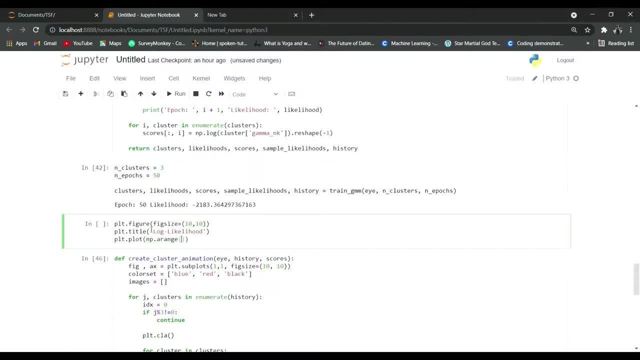 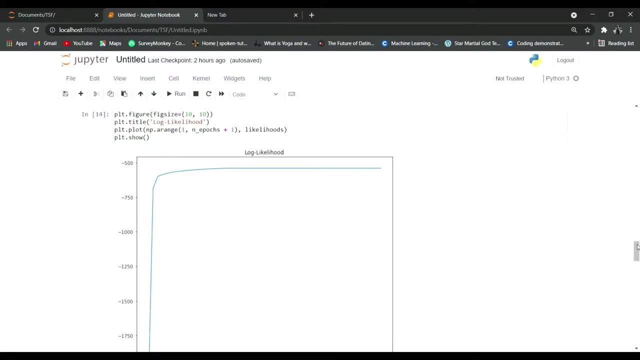 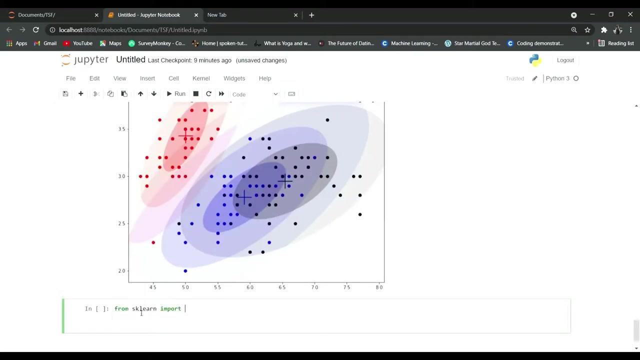 The likelihood graph shows us the probability of observed data under the model, And let's now test if our calculations are correct. We are going to use SKLearn's GMM implementations to check for the parameters and probabilities. I'm going to create a new gráfic to check the parameters.